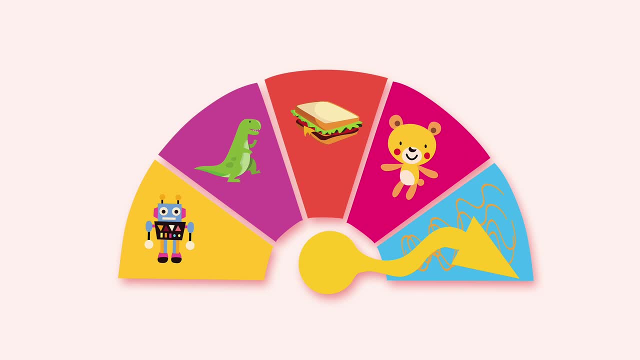 can make it through all five levels today. For every level you do, you get a gold star chime like this: So if you do all five levels, you'll get five gold star chimes, Woo-hoo. Now, if you are super awesome at being floppy and you do make it to level five, let me tell. 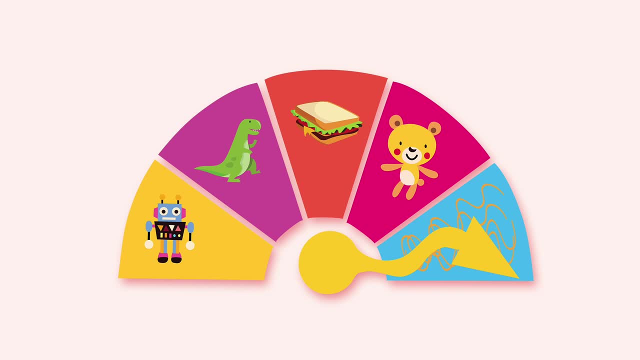 you, you will have reached the top flop spot. What do you think? Are you ready to see if you can do it? I wonder if you'll be able to do all five. Let's try it out and see. We begin at level one. 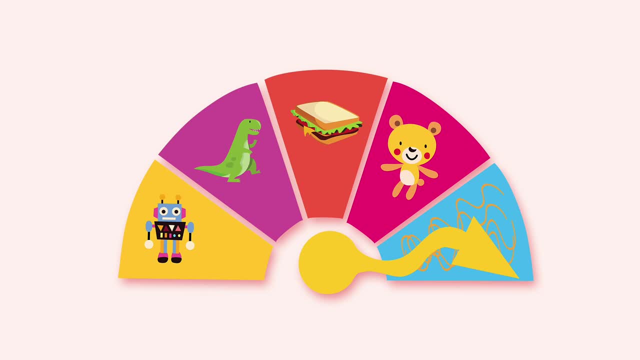 Make yourself as floppy as a robot. Wow, that's not floppy at all, is it? Are you doing it? I'm about as unfloppy as it gets. Everything is super stiff and rigid, Level one complete. Yay, we did it. Well done you. 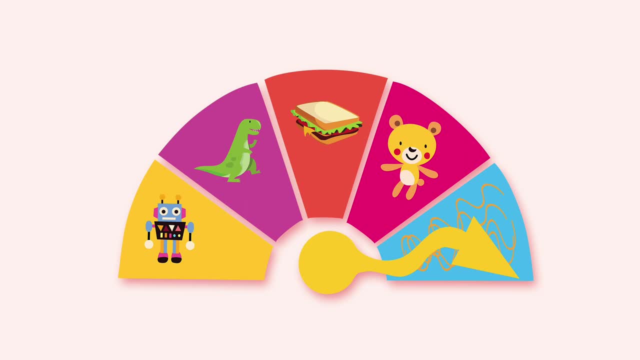 Thank you. Now let's go for level two. Make yourself as floppy as a dinosaur. Goodness, still not very floppy. How about you? I feel like I have claws on the ends of my fingers and toes and lots of teeth in my mouth. 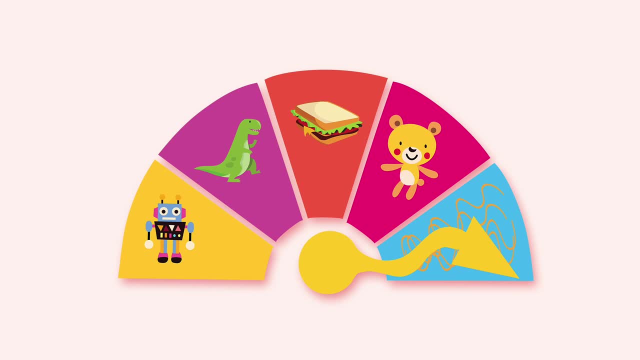 Level two: complete Good work. Next one, Level three: Make yourself as floppy as a sandwich A sandwich. Well, I suppose sandwiches are more floppy than dinosaurs and robots. Let's try it. It feels a lot less tense, don't you think? But still a bit stiff, so that all the fillings don't fall out of the sandwich. 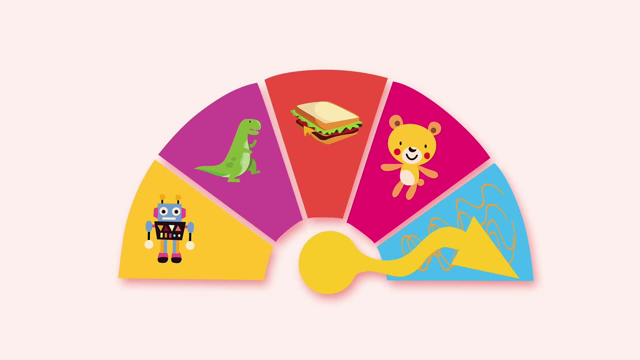 Level three: complete. Level three, complete. Yes, you did it On to the next one. now Level four: Make yourself as floppy as a teddy- Ah, nice, A teddy. When I think of my teddy, I remember how floppy he is: his arms and his legs and a wobbly head. 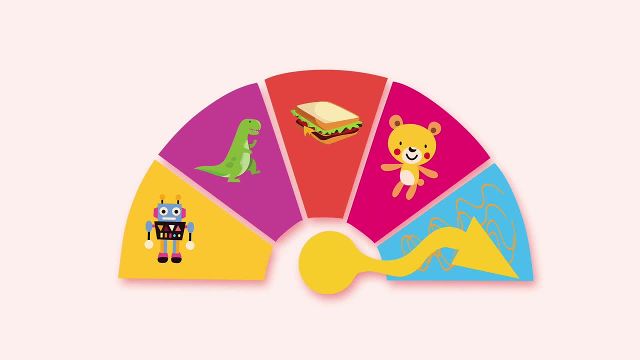 When I do it with my body, it feels pretty floppy to me. How about you? Level four complete. We're nearly there. This is great. We are doing so well on the Flop-O-Meter so far. I wonder if we can be any more floppy. 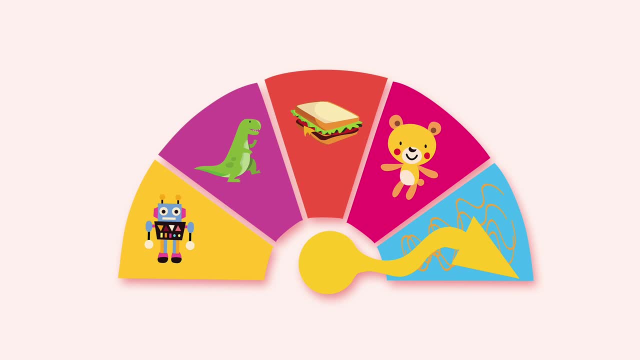 Only one way to find out. Let's go for the big one. Level five: Make yourself as floppy as cooked spaghetti. Oh, that's really floppy. I'm making my legs and arms as floppy as can be. In fact, I'm making my body really floppy too, and my face. 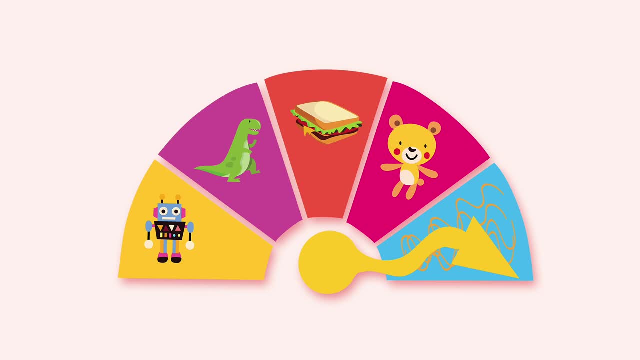 Let's see if we can stay floppy enough to get our final fifth gold star, chime. Yay, we did it. We reached level five. Would you like to score some extra bonus flop points? The best cheat for the extra flop points is to close your eyes. 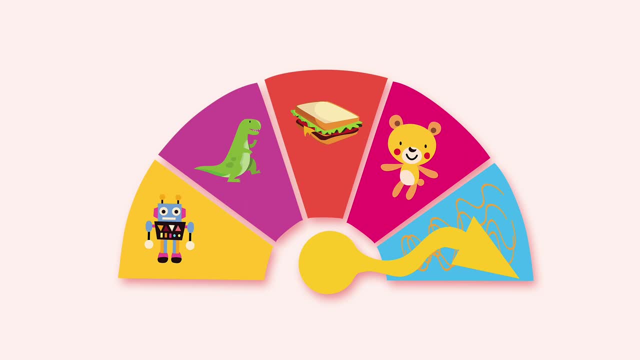 Make yourself like the cooked spaghetti again and just breathe slowly In through your nose and out through your mouth, And again In through your nose. In through your nose And out through your mouth. That's it Well done, Wow. did you hear that? That was the Flop-O-Meter telling you that you're the new highest scorer? Fantastic. 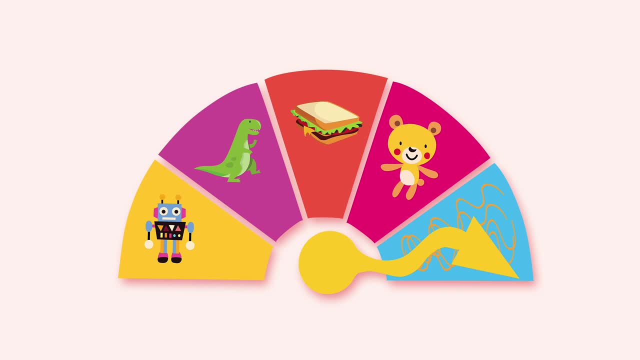 Now you know about the floppiness levels, You can help your mind get super ready for our peace outs. Isn't it amazing how your body can affect your mind? But now you know about the special level of Flop, You can use it whenever you need. 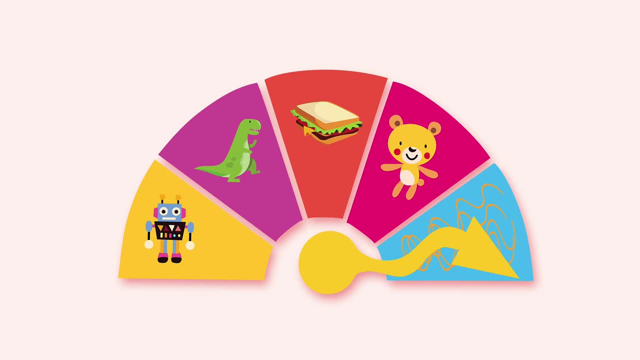 You did so well with the Flop-O-Meter And I hope you found it fun. I did. I hope it helps you too. So the next time you want to think clearly or enjoy peace out, you know exactly how to relax your body.